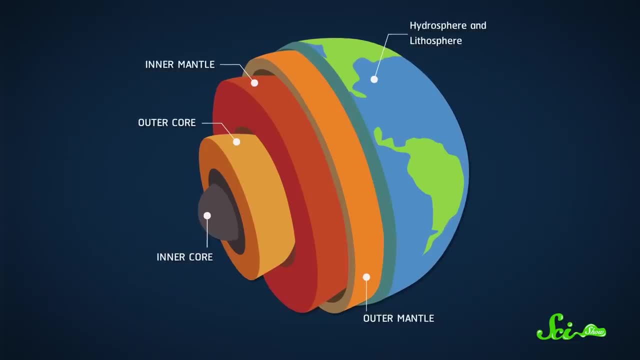 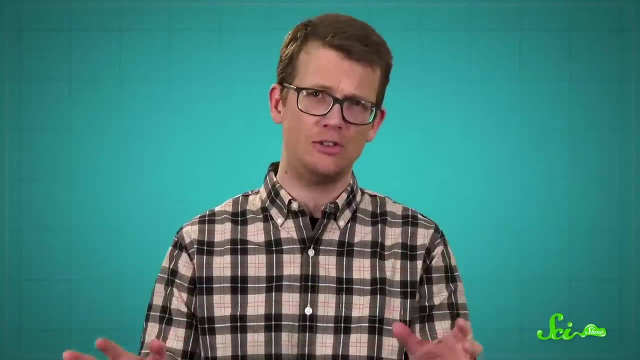 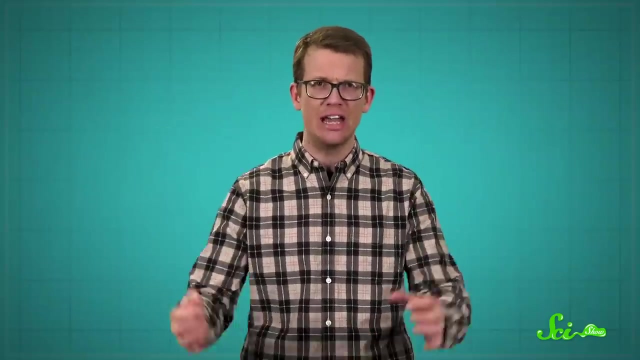 and a solid metallic inner core, with even more transitions and subdivisions in between. But figuring all this out has involved some inventive thinking across multiple scientific disciplines and it's taken scientists to some surprising places- The ways we have peered inside our planet. 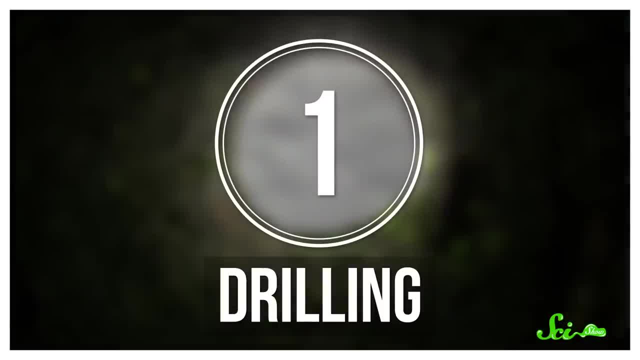 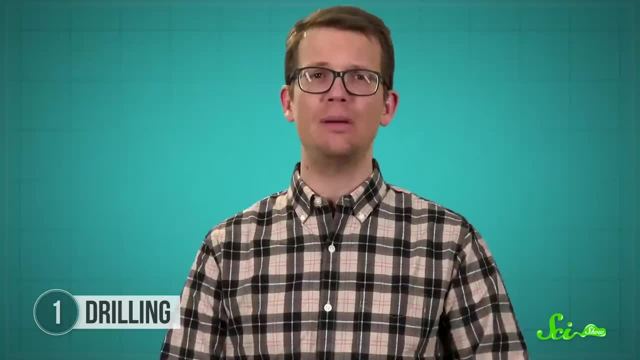 Let's start with the obvious one: just digging a big hole. No one has been able to dig down to the mantle yet, but that doesn't mean people haven't tried. In 2005,, for example, an international group of researchers called the 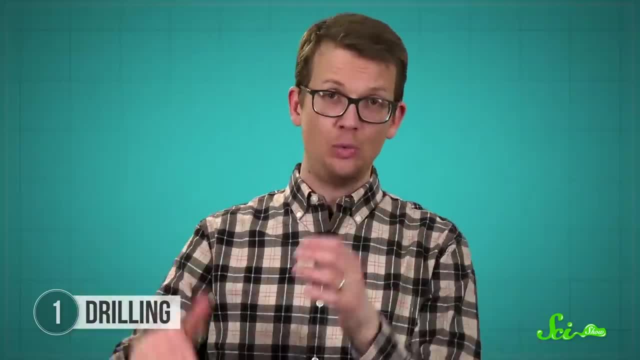 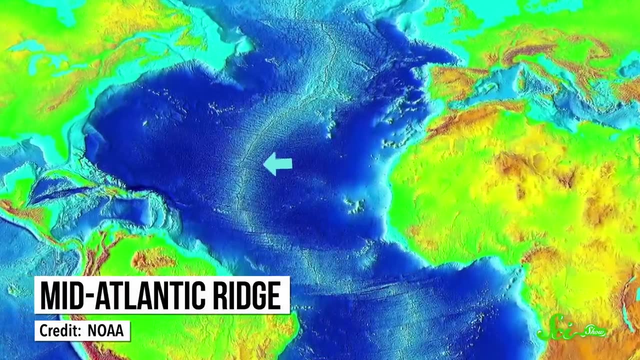 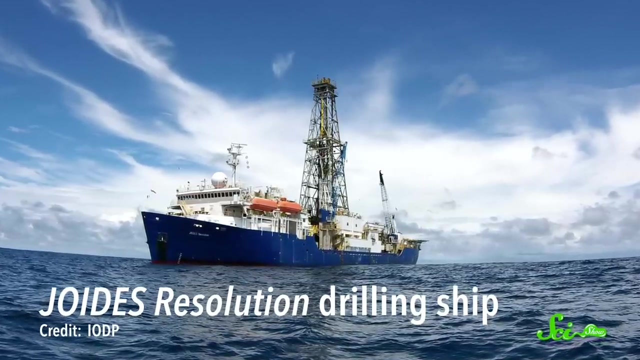 Integrated Ocean Drilling Program set out to reach the crust-mantle boundary. To do this, they targeted a thin point of crust located on the floor of the North Atlantic Ocean And in the end, they weren't Able to get there after drilling down for more than 1.4 kilometers. 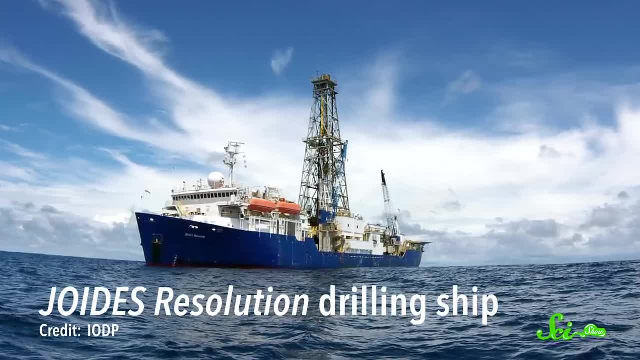 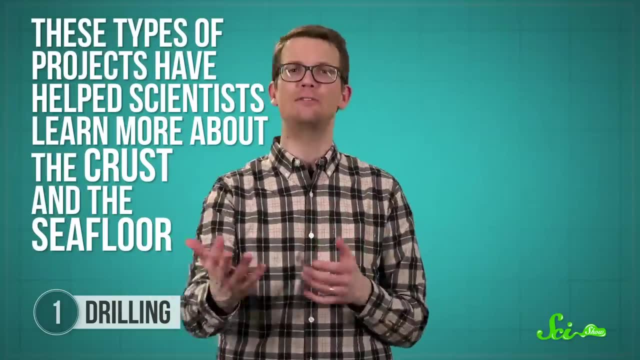 they missed the thin patch by only about 300 meters, Even if they haven't successfully made it through. these types of projects have helped scientists learn more about the crust and the sea floor, such as the unique microbial communities we can find down there. 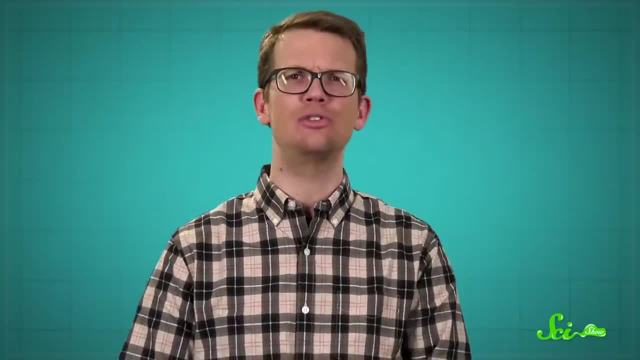 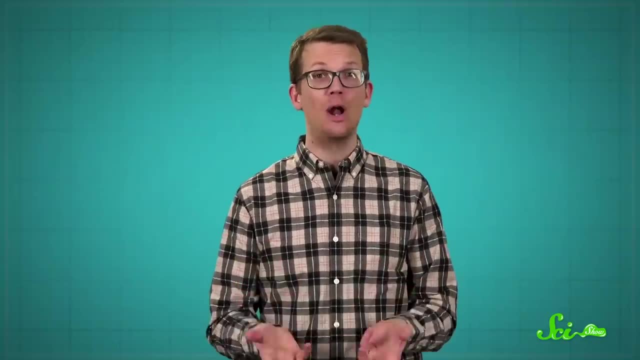 And we haven't quite given up on drilling yet. A team of Japanese researchers, for instance, is looking at trying their hand somewhere near Hawaii in the near future. A simpler idea is to just study rocks and geological activity right here on the surface. 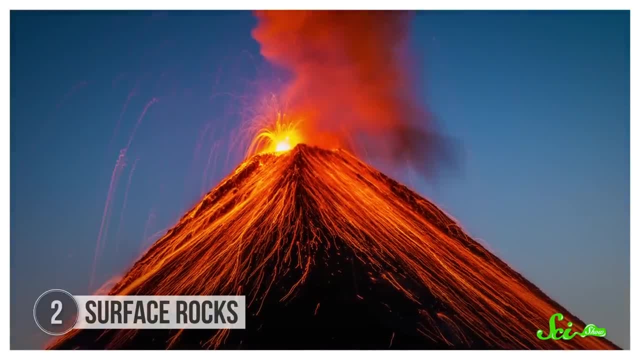 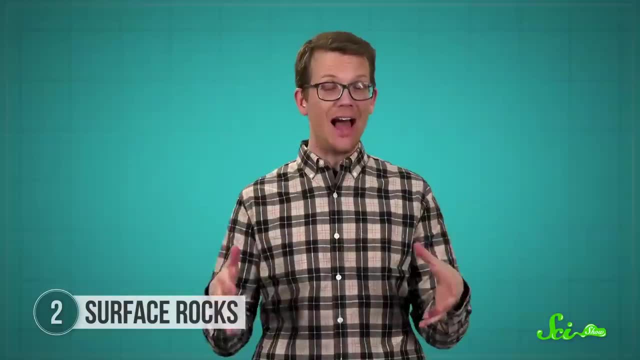 Studying volcanoes and fault lines, for example, can teach us more about plate tectonics, where hotspots in the mantle might be and how magma reservoirs form underneath volcanoes. And there's a lot we can learn just from looking at rocks, especially older ones. 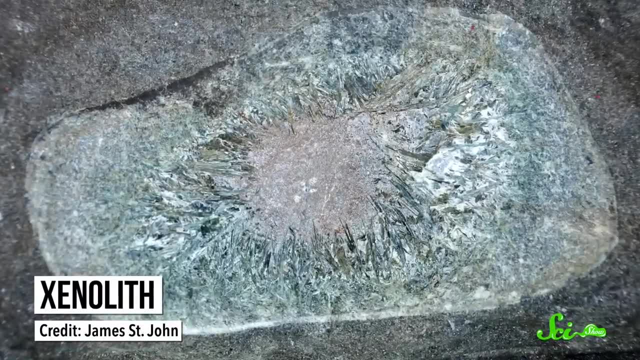 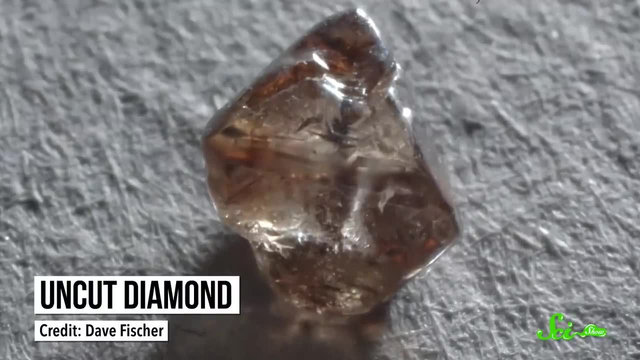 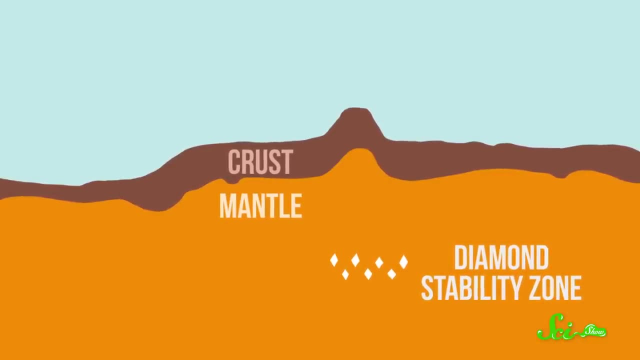 Xenoliths are parts of Earth's mantle brought to the surface trapped inside other bits of volcanic rock. The most informative and spectacular type of xenolith are diamonds. Diamonds form only under very specific conditions, at depths of 150 kilometers or more in the upper mantle. 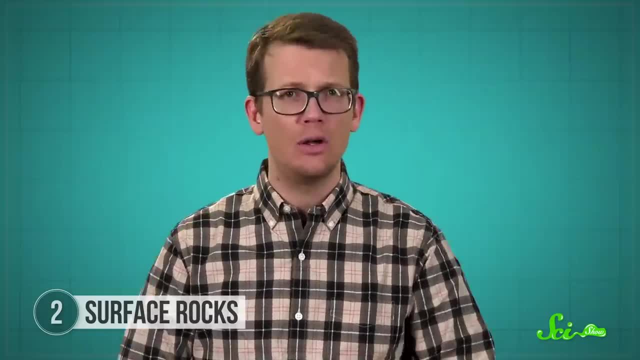 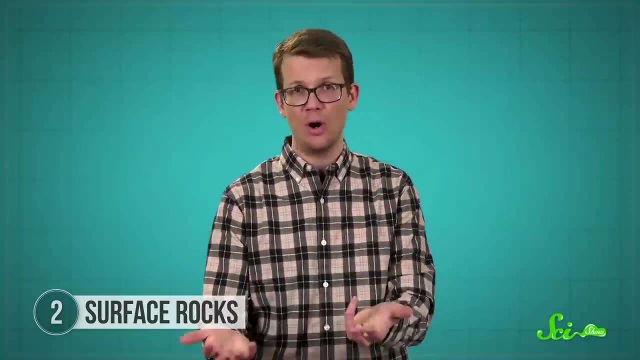 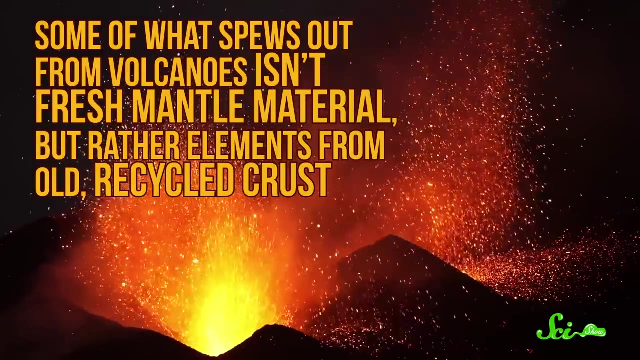 So anything trapped in the diamond, or anything that comes up alongside it, must have come from at least that far down. Scientists can also examine the chemical makeup of ancient rocks. That's revealed that, among other things, some of what spews out from volcanoes isn't fresh mantle material, as you might expect. 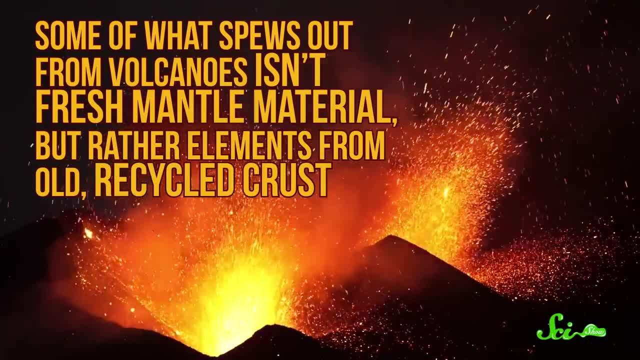 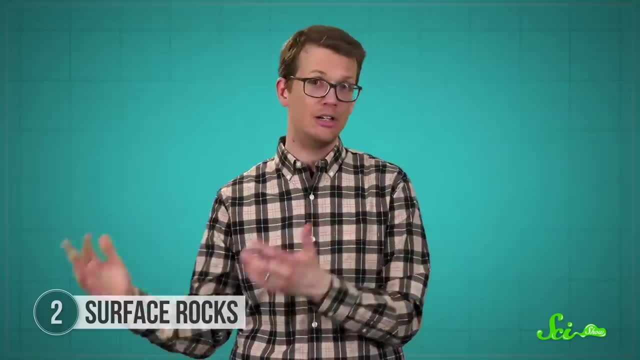 but rather elements from old, recycled crust. In 2016,, researchers measured the ratio of magnesium isotopes in solidified lava from the French island of Martinique. Then they compared that to the ratios previously seen in other crust and mantle material. 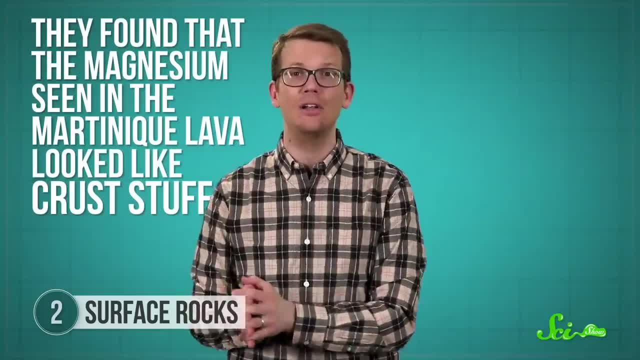 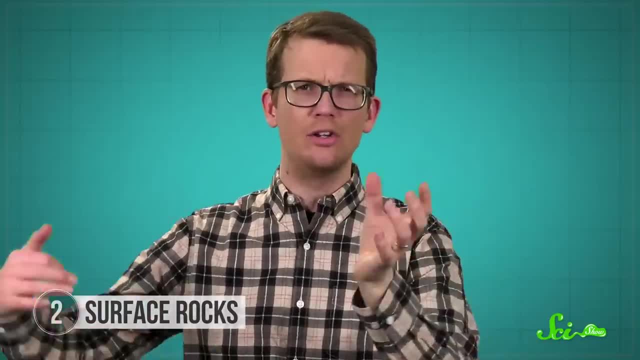 They found that the magnesium seen in the Martinique lava looked like crust stuff. The team thinks that certain elements might get squeezed out of the rocks along with water to travel towards the surface as bits of old crust sink, In other words, bits of surface. 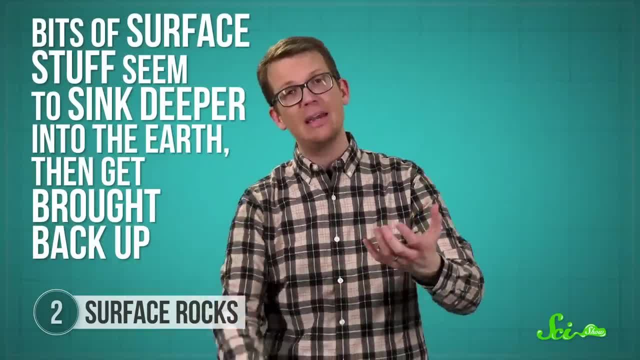 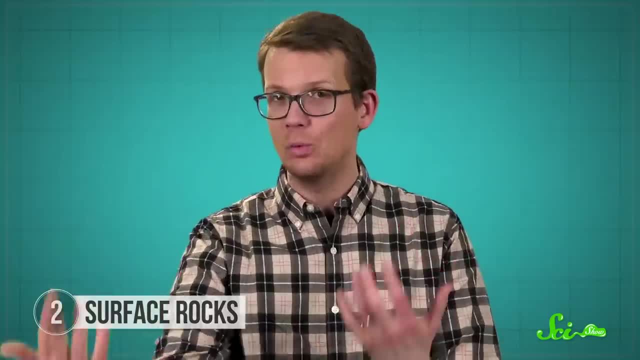 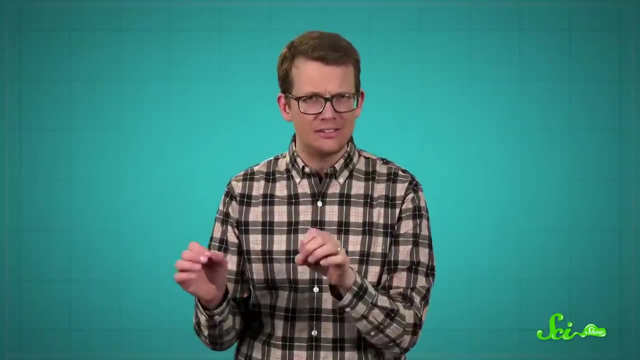 stuff seemed to sink deeper into the Earth and then get brought back up. Understanding how these fluids travel could help us better understand how volcanoes and earthquakes work. Digging, looking at rocks and studying volcanoes is all pretty hands-on stuff, but there are also ways to look inside the Earth without heading into the field. 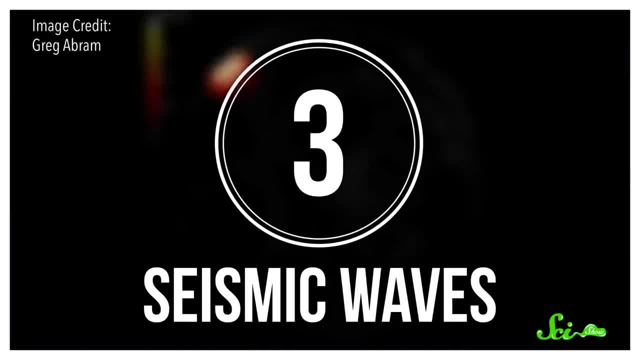 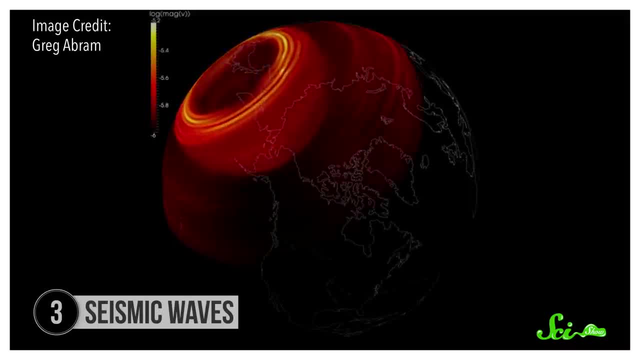 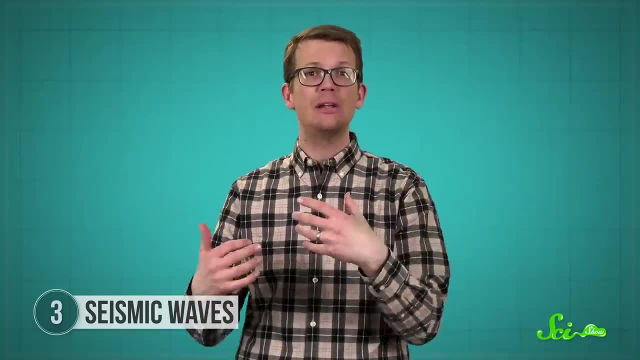 such as using seismic waves. These are the vibrations created not by us but by earthquakes that spread through the Earth like ripples across the Earth. These ripples are called seismic waves, or seismic waves across a pond. Different densities of rock bend or reflect those waves. 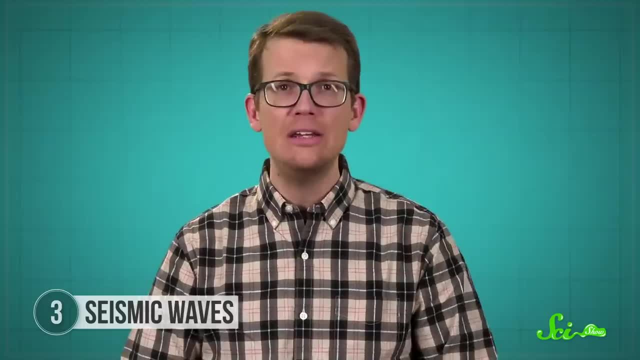 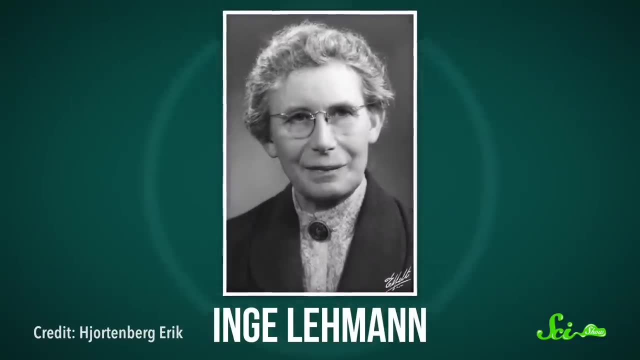 By analyzing the patterns, researchers can make inferences about the shape of things underground. This approach was key to one of our first big breakthroughs in understanding the Earth's interior. In 1929, Danish seismologist Inge Lehmann was examining seismic waves. 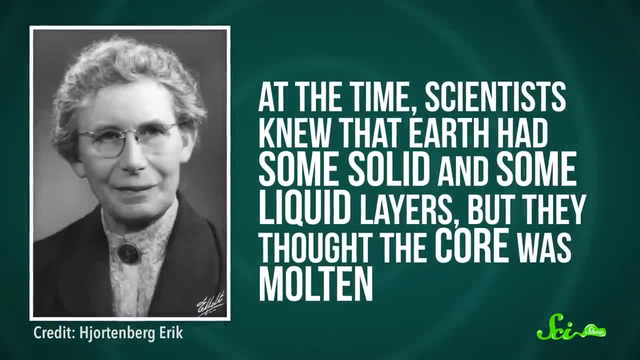 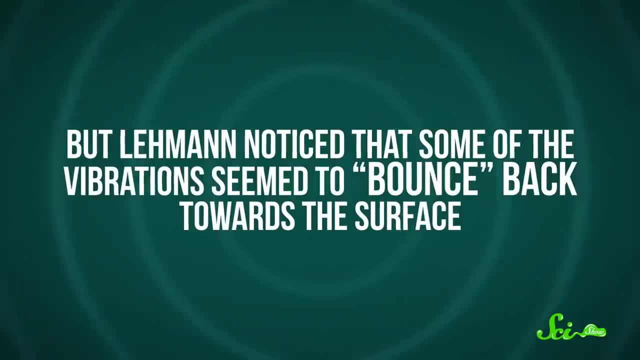 At the time, scientists knew that Earth had some solid and some liquid layers and that, in order to identify these layers, the waves from an earthquake should spread out smoothly from its epicenter. But Lehmann noticed that some of the vibrations seemed to bounce back toward the surface. 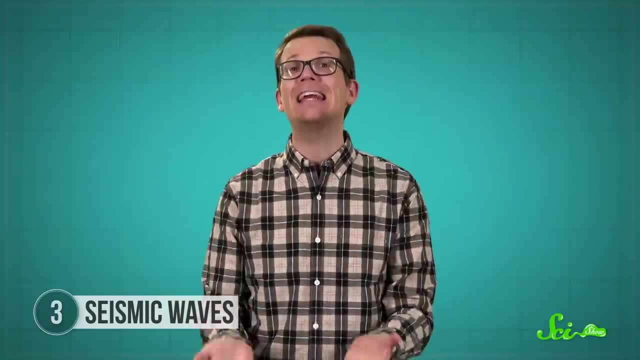 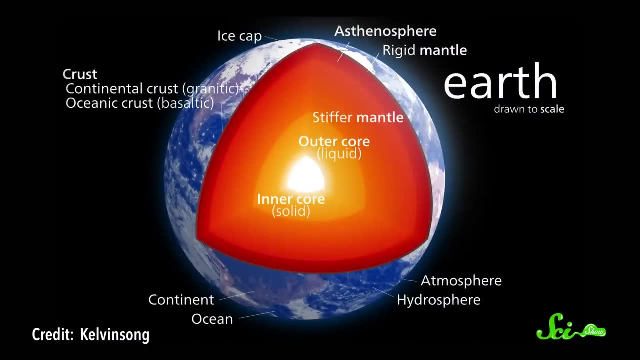 The only explanation she figured would be that they were reflecting off something big and rigid at the center of the Earth. We now know that that thing is our planet's solid inner core. Today, we are still using seismic waves to learn more about the Earth's interior. 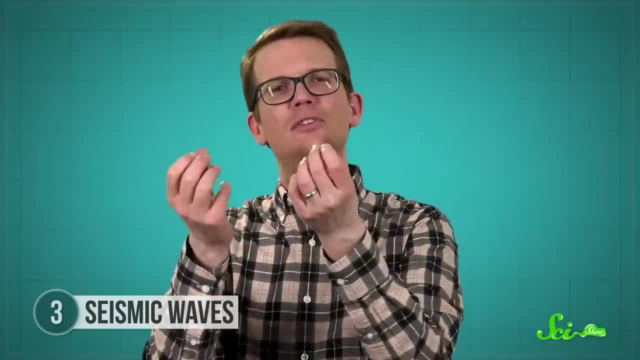 In 2019,, for example, scientists found a kind of seismic wave that was like the Earth's interior. In 2019,, for example, scientists found a kind of seismic wave that was like the Earth's interior. It was a kind of iron snow falling from the outer core towards the inner one. using seismic wave data. 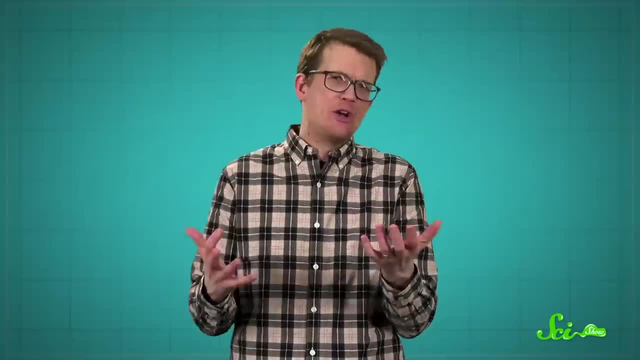 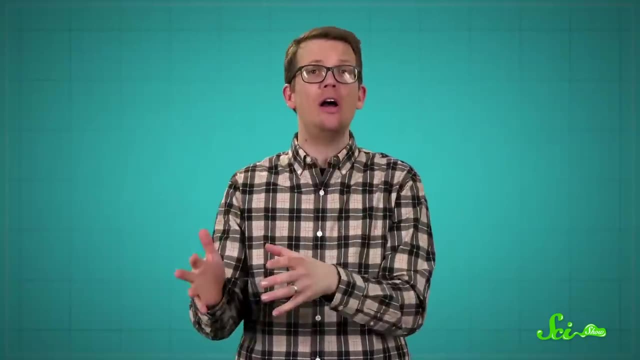 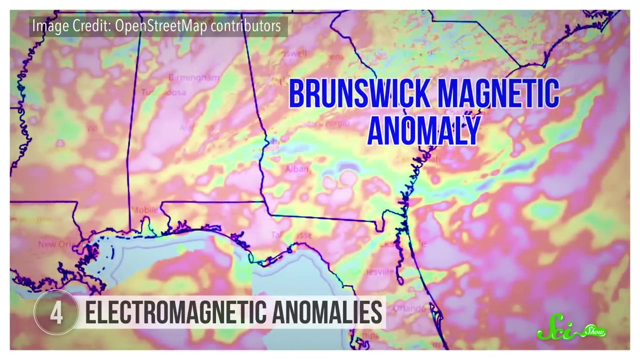 We can also learn a lot from noticing when things get weird. Irregularities in the planet's properties happen for a reason, and sometimes that points toward a cause that we can't actually see. For instance, there is a line known as the Brunswick magnetic anomaly. 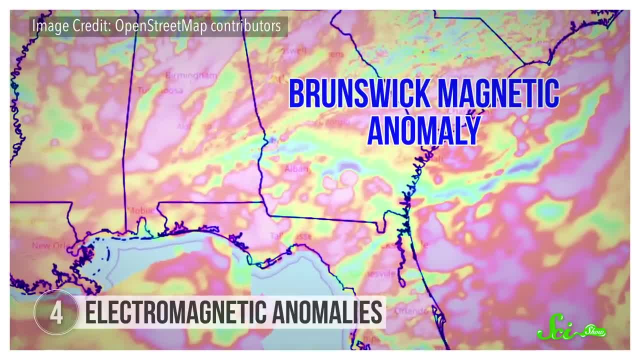 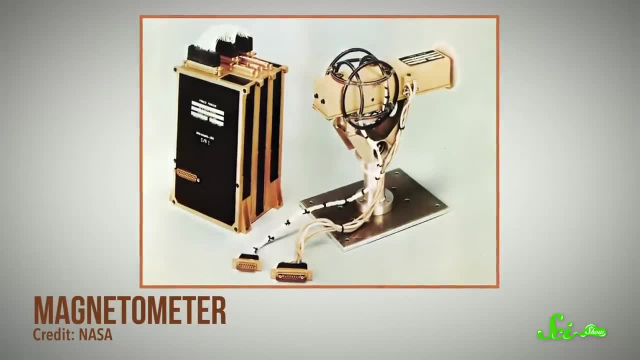 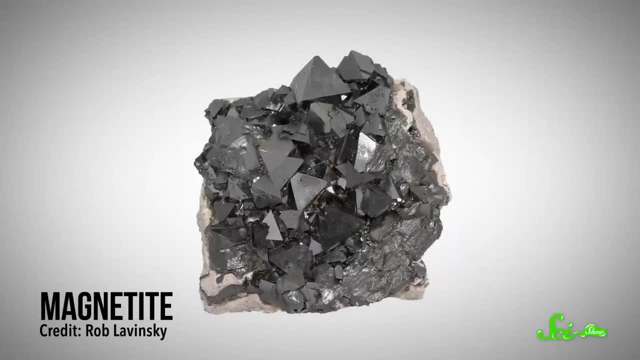 that runs through Alabama and Georgia, where the Earth's magnetic field seems unusually weak. Scientists can map this thanks to magnetometers, which measure the strength of a magnetic field. Magnetic anomalies can be caused by the composition of rock in an area. A streak of magnetite ore which contains iron may have an unusually strong magnetic field. 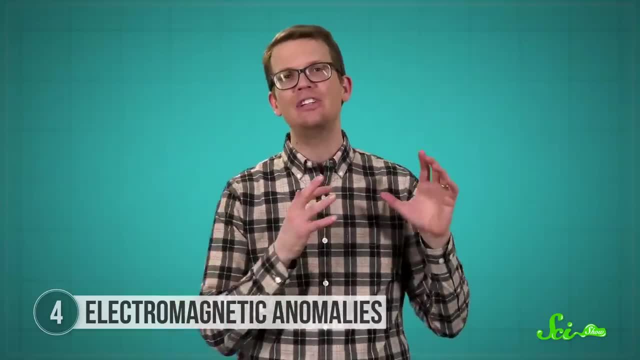 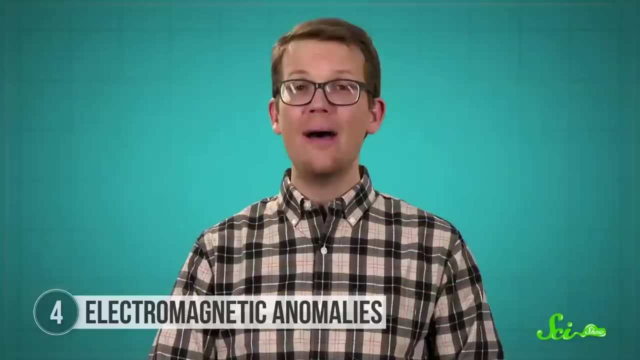 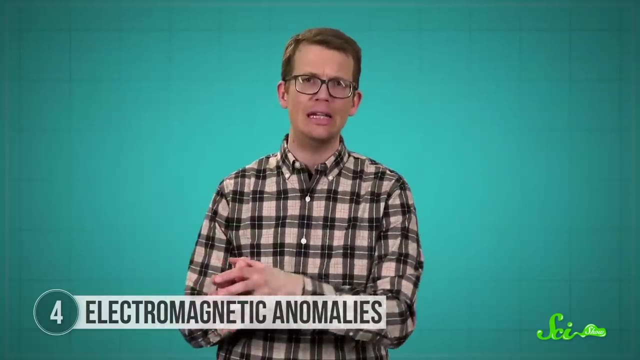 On the flip side, a particularly weak field might mean that there's a significant lack of magnetic material. Sedimentary rocks like sandstone often contain relatively little metal. These anomalies can also teach us about geologic history. For example, a 2014 study suggested that the Brunswick anomaly was due to rock left behind. 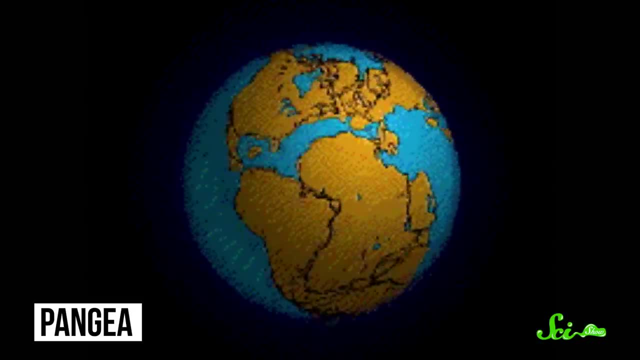 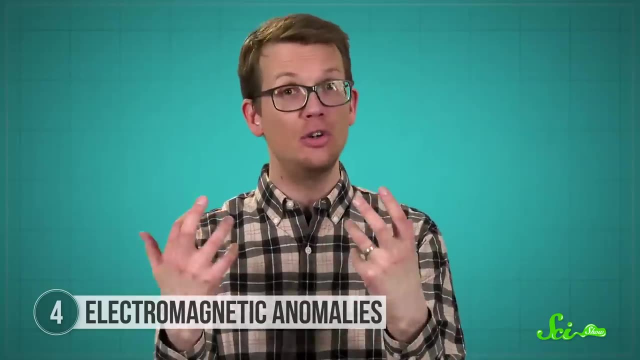 millions of years ago, as the supercontinent Pangea split up, separating North America from Africa. We can also look for anomalies in how well the crust or upper mantle conduct electricity. Earth's magnetic field varies naturally over time and changing magnetic fields create 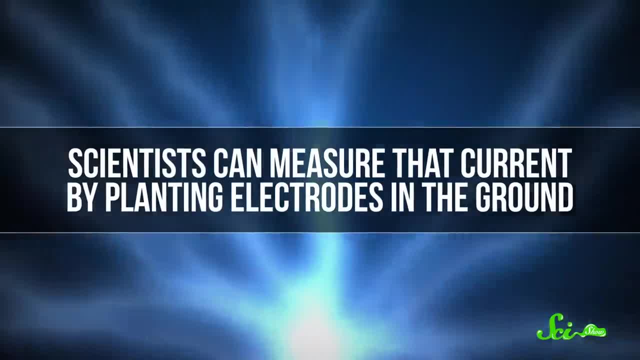 currents of electricity. Scientists can measure that current by planting electrodes in the ground. Then they can measure the magnetic field. They can measure the magnetic field by planting electrodes in the ground. Then they can measure the magnetic field by planting electrodes in the ground. 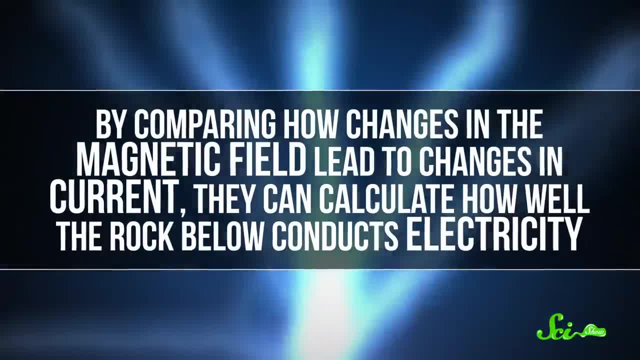 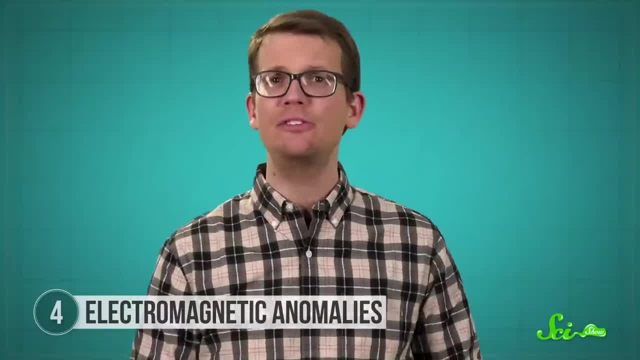 Then they can measure the magnetic field by planting electrodes in the ground. Then by comparing how changes in the magnetic field lead to changes in current, they can calculate how well the rock below conducts electricity. Depending on how things are set up, this technique can peer hundreds of kilometers below the 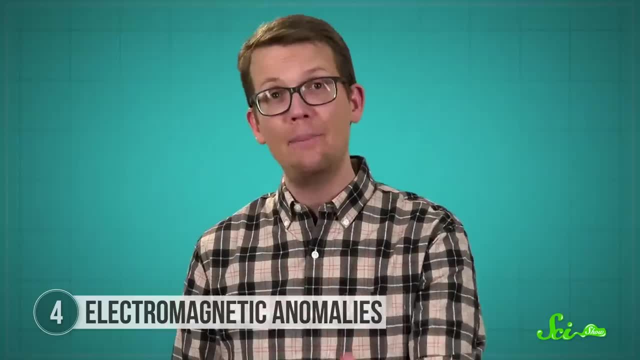 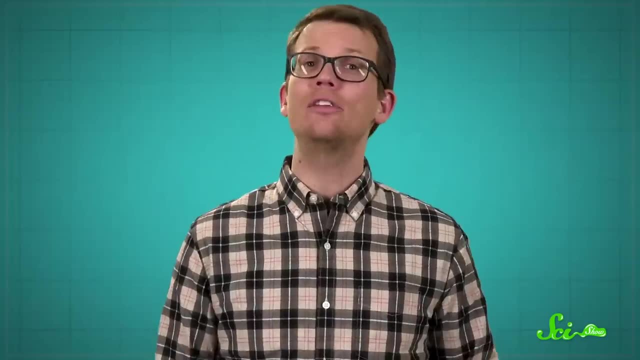 surface, revealing properties like the temperature and even composition of the material down there. It can also help researchers calculate how much water is trapped in the rock. In fact, one study found that there might be as much water in the mantle as in all of. 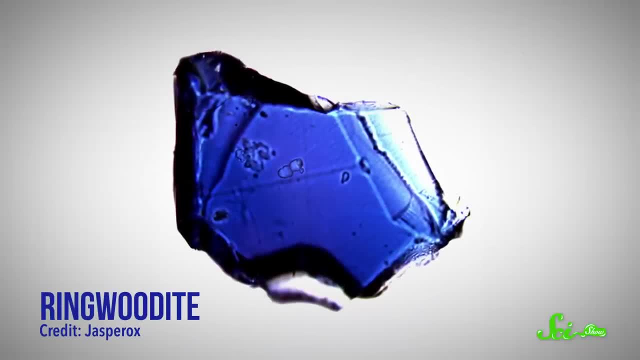 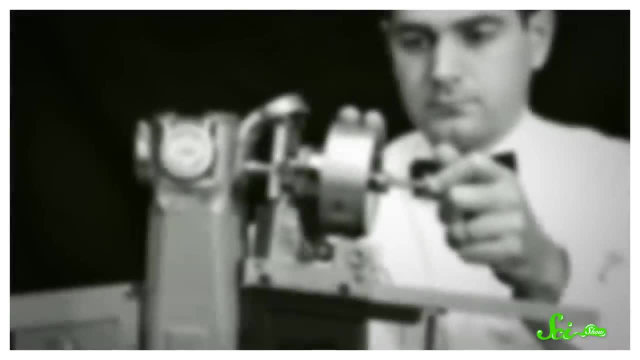 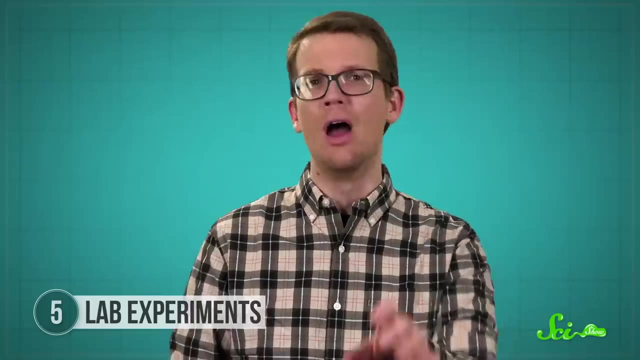 the oceans. So far, we've looked at real measurements in nature, but figuring out what those mean often relies on scientists' models and lab experiments. The pressures and temperatures deep within Earth can be extreme, resulting in physics and chemistry that behave differently than up here on the surface. 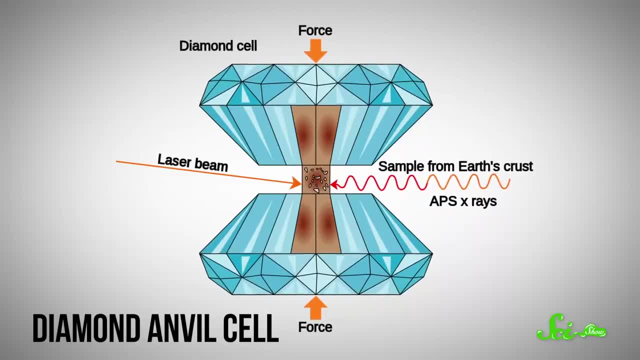 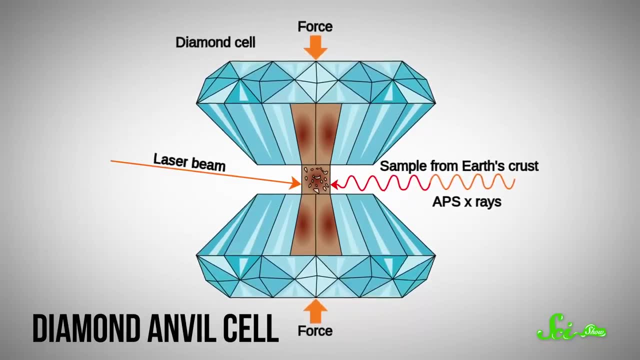 One tool scientists use is the diamond anvil cell, which consists of two small, flawless diamonds. Ground to precipitate. The diamond is made up of precision points and mounted on pistons. Since pressure is force divided by area according to the math, when the pistons apply their 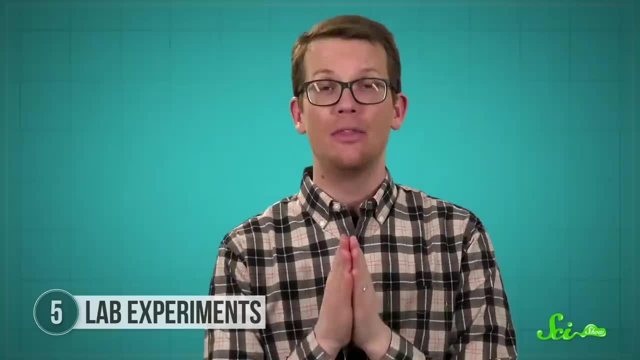 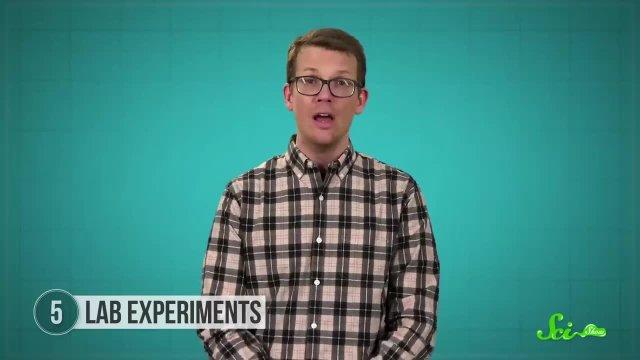 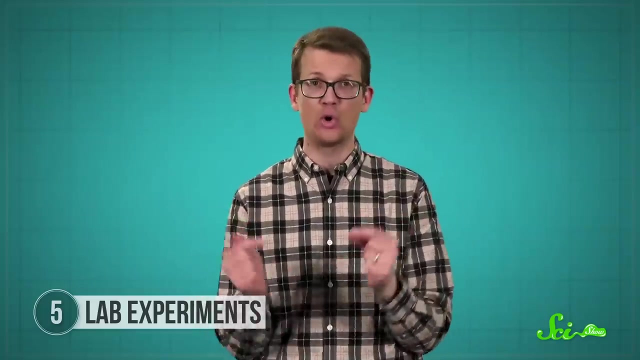 huge force to the tiny points of the diamonds. the pressures can be ridiculous. In 2009,, for instance, scientists reported subjecting an iron alloy to 200 billion pascals of pressure, more than half of what it would be inside the inner core. 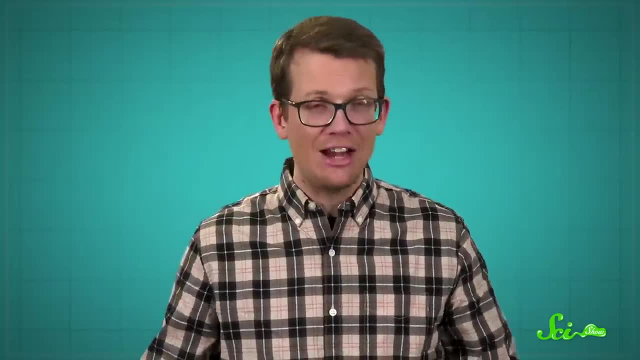 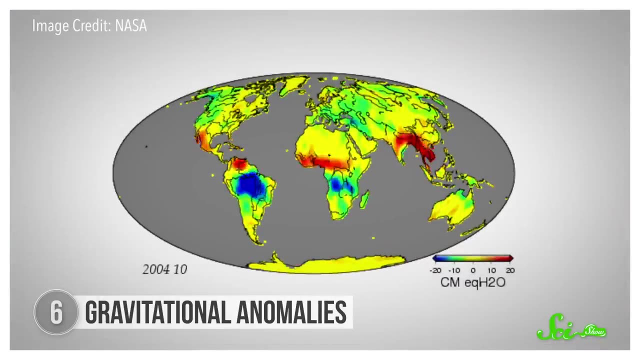 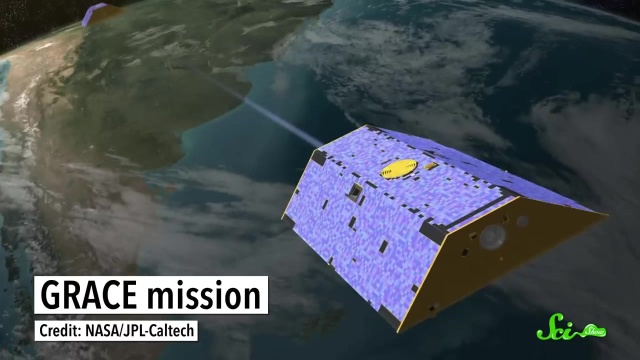 Amazingly, to find some of the planet's interior anomalies. we had to find a way to find them. We actually have to go to space. This is especially true for one particular kind—gravitational anomalies. From 2002 until 2017, NASA's GRACE mission used two spacecraft more than 500 kilometers. 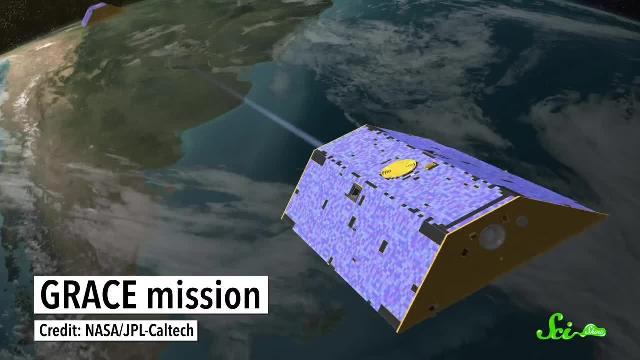 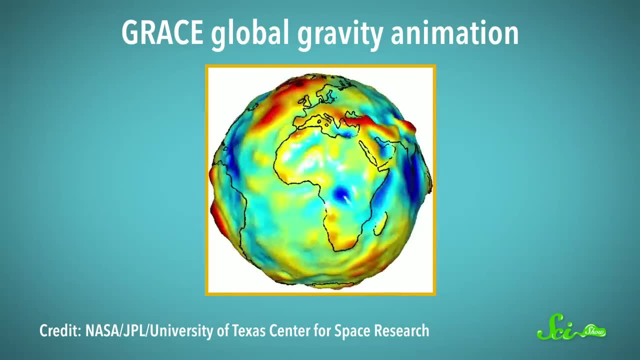 above the Earth's surface to map out fluctuations in Earth's gravitational field. The result was maps like these that show where gravity is oddly strong or weak. If you think back to high school physics, you might remember that the most powerful and powerful object in the universe is the Earth. 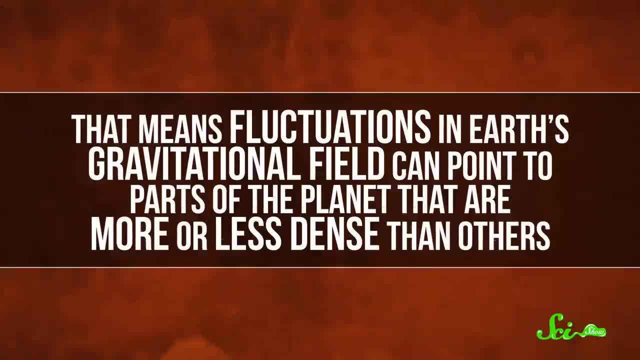 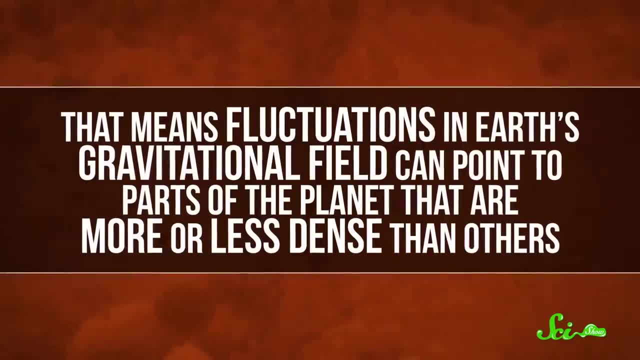 But remember that the more mass something has, the more gravity it exerts. That means fluctuations in Earth's gravitational field can point to parts of the planet that are more or less dense than others, And since the crust, mantle and core are made of stuff with different densities, scientists 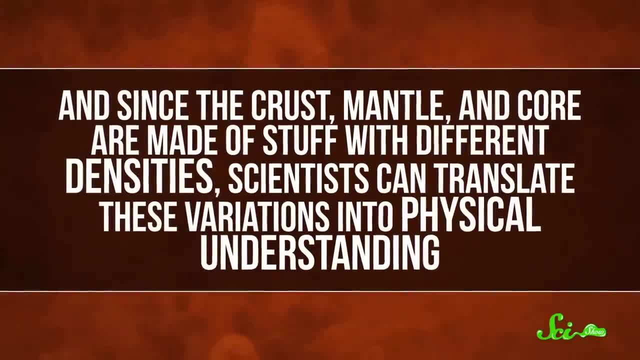 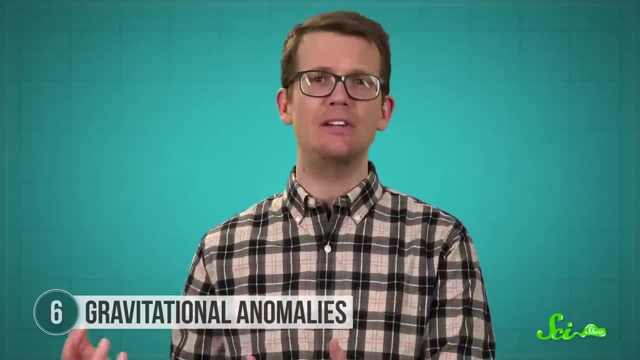 can translate these variations into physical understanding. For example, if the crust in an area is known to be less dense than the material in the mantle, weaker gravity might point to a bit of friction. That's why the Earth's gravitational field can point to parts of the planet that are 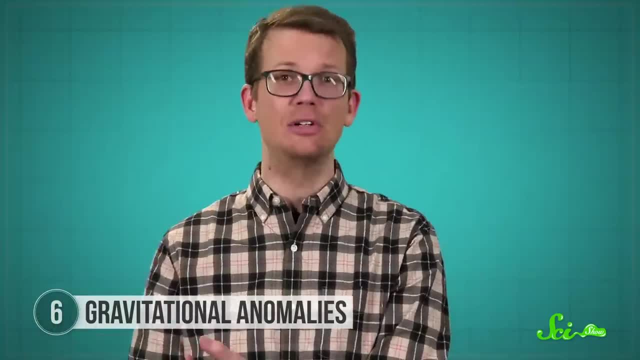 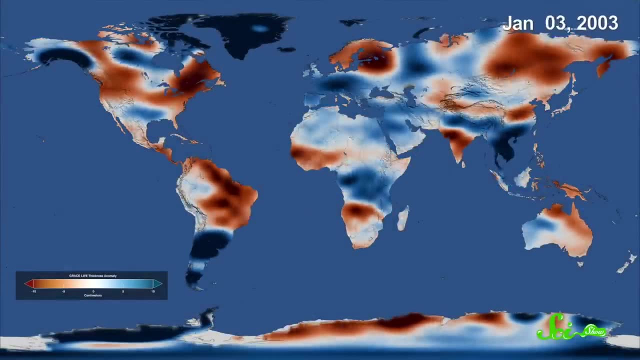 more or less dense than others. That's why it's called the crust getting sucked down into the mantle. The precision of these measurements can get even more specific than that, though. GRACE has also helped map the disappearance of aquifers and measure the rate at which. 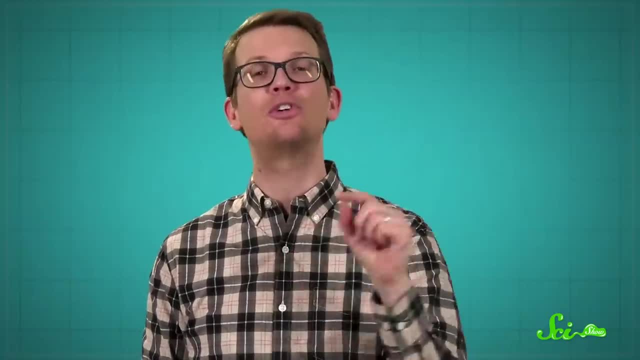 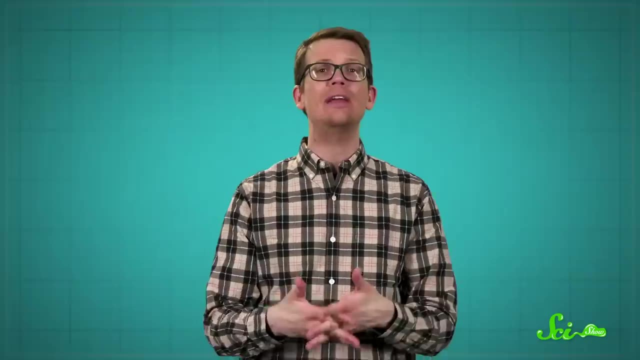 ice sheets are melting, And this is wild. Scientists have even used ground-based gravity measurements to locate abandoned mine shafts in England. Finally, not only can we examine the interior of Earth by going to space, we can also let space come to us. 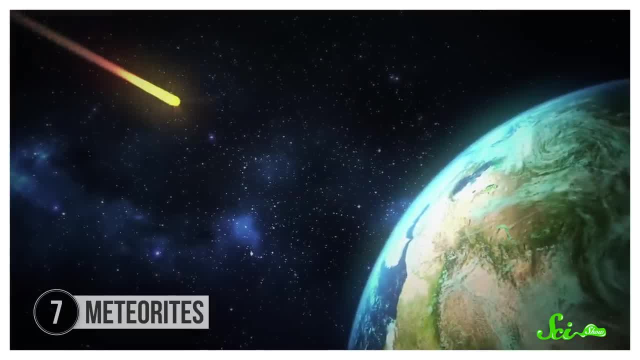 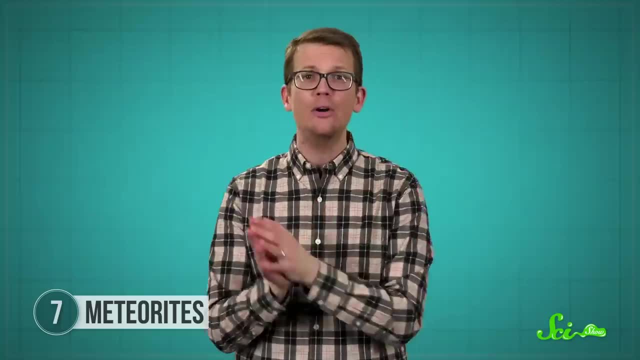 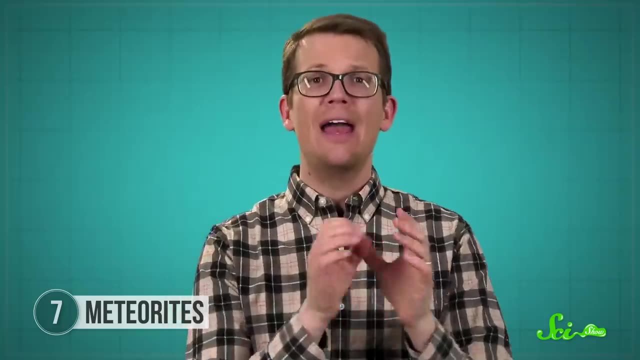 Meteorites can represent the solar system's building blocks, the same stuff planets like Earth formed out of billions of years ago. By studying them, scientists can learn about the Earth's starting conditions and how things have changed over time. For instance, in 2005,, a group narrowed down the date that early Earth's crust turned. 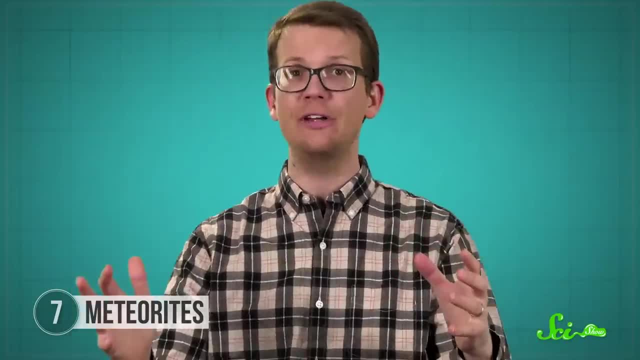 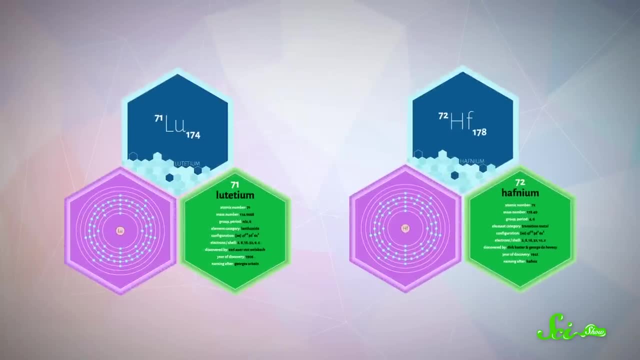 from a sea of molten rock into an actual solid surface. They did it by examining the ratio of a radioactive isotope of the element lutetium to the ratio of lutetium to the element. it decays into hafnium in samples collected from both a. 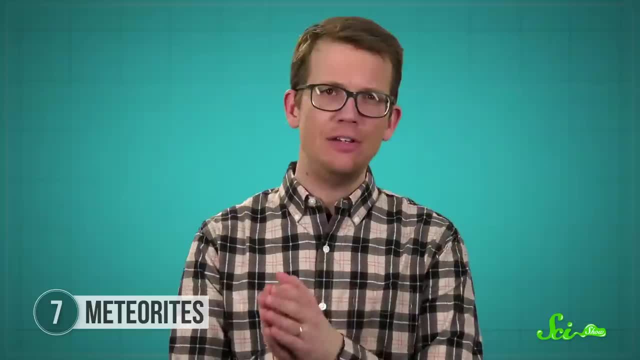 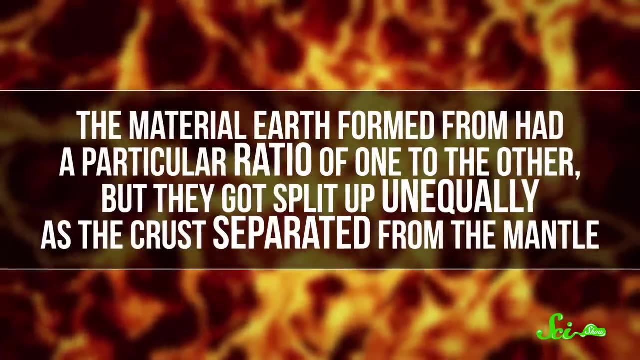 meteorite and the Earth's oldest rocks. Both of these elements were present on Earth way back when the planet's surface was still molten. The material Earth formed from had a particular ratio of one to the other, but they got split up unequally, as the crust separated from the mantle. 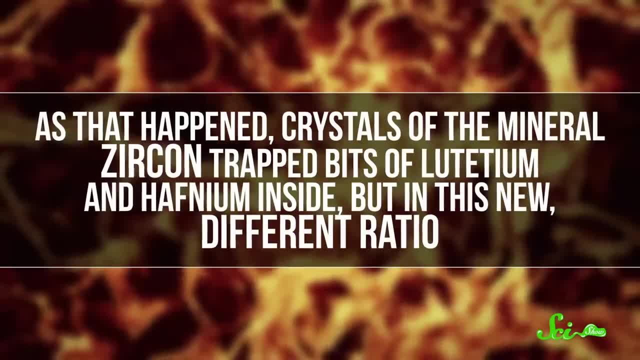 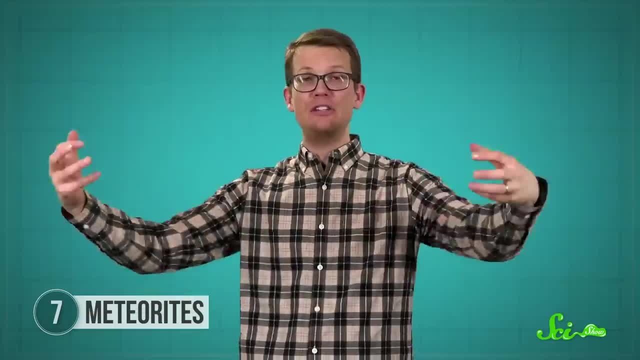 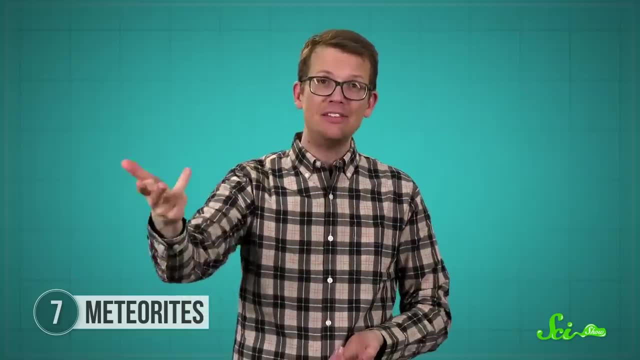 As that happened, crystals of the mineral zircon trapped bits of lutetium and hafnium inside. But There was a new, different ratio. All the stuff that didn't form into Earth stayed in space with the original mix. Billions of years later, bits and pieces arrived, trapped inside meteorites. 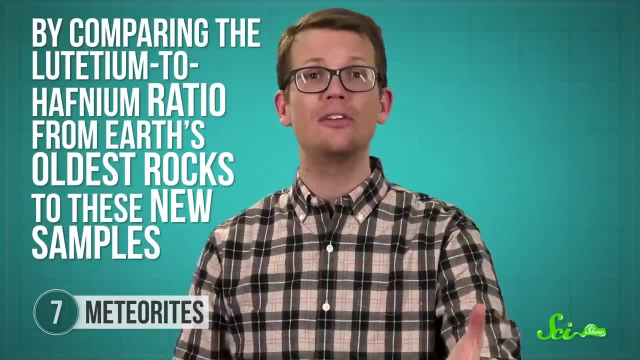 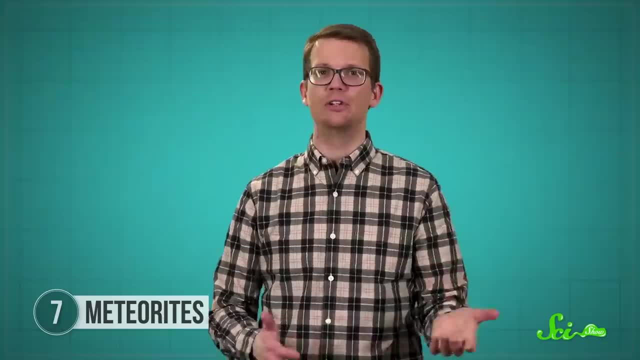 By comparing the lutetium-to-hafnium ratio from Earth's oldest rocks to these new samples from space, scientists were able to work out when the crust must have formed. Their answer- around 4 billion years ago- suggests the crust started solidifying less. 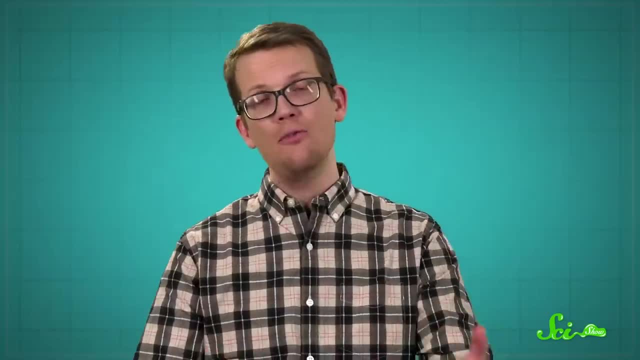 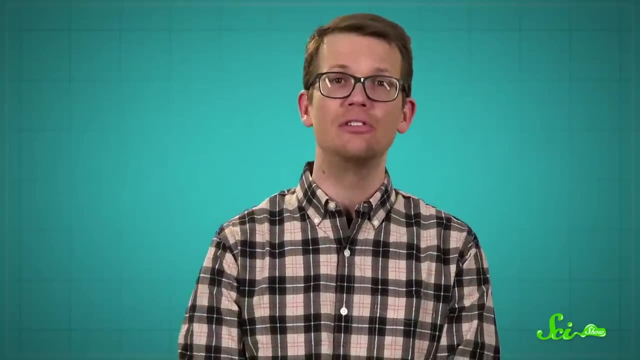 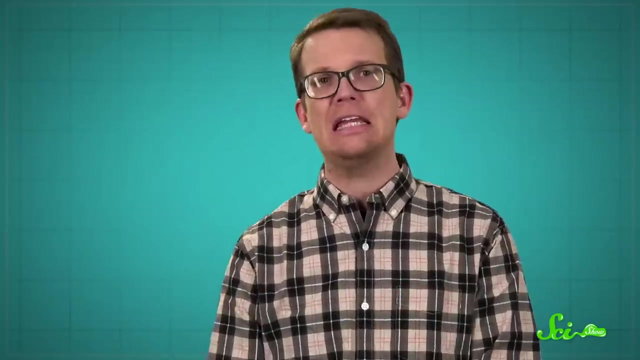 than 100 million years after the Earth itself. So yeah, unfortunately the Earth isn't see-through, And yet, thanks to a range of careful, often clever, observations, we can still picture, to a remarkable degree, the complicated roiling world beneath our feet. 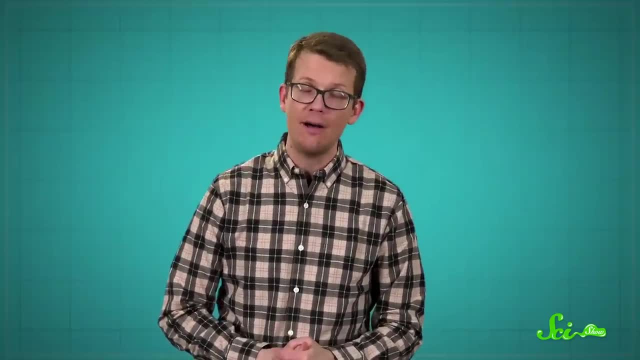 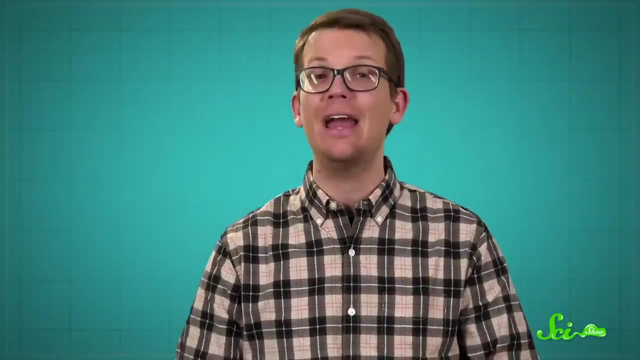 Thanks for watching this episode of SciShow, which was brought to you with the help of our amazing patrons. Patrons don't just help us do what we do here. They also get access to fun perks like blooper reels and our patron-only Discord. 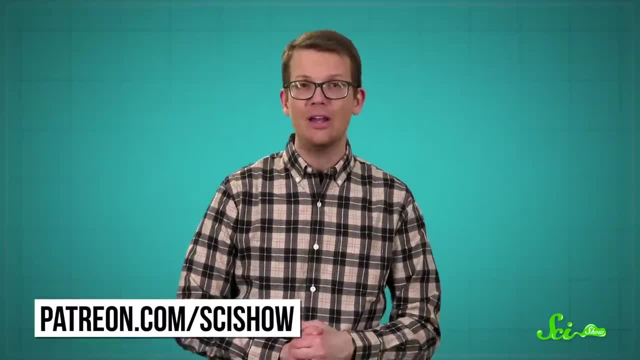 If you're interested in joining up and helping out, please subscribe to our channel And, to help us exist, check out patreoncom slash scishow.